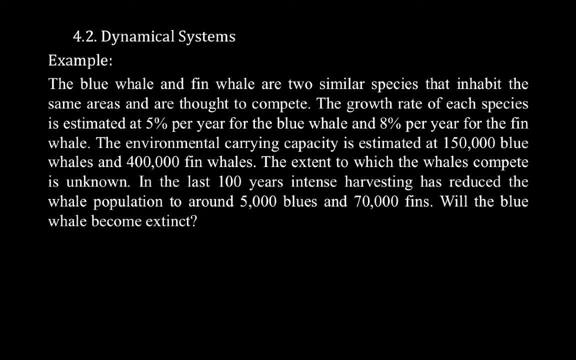 species that inhabit the same area. The growth rate of each species is estimated at 5% per year for the blue whale and 8% per year for the fin whale. The environmental carrying capacity is estimated at 150,000 blue whales and 400,000 fin whales. The extent to which the whales compete is unknown. 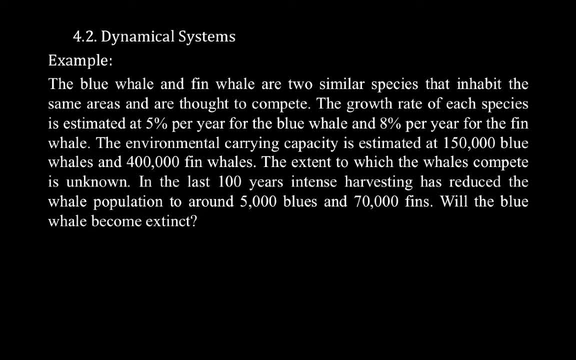 In the last 100 years, intense harvesting has reduced the whale population to around 5,000 blues and 70,000 fins. Will the blue whale become extinct? We are going to follow the five-step method As we know. the first step: 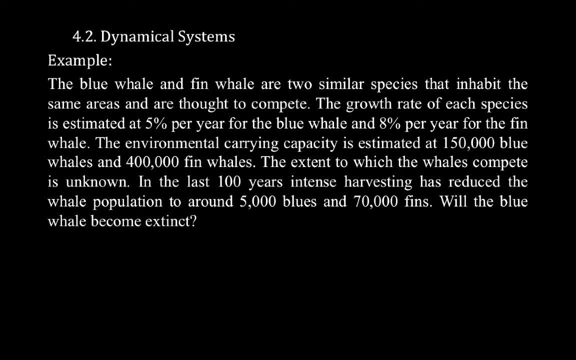 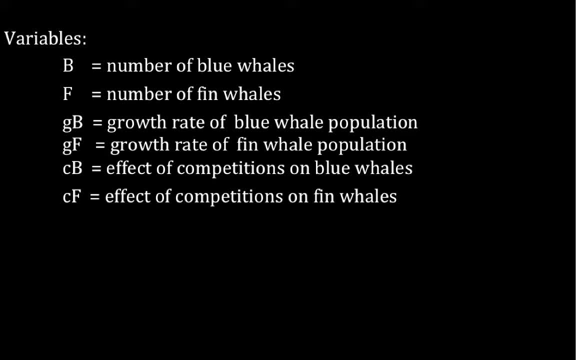 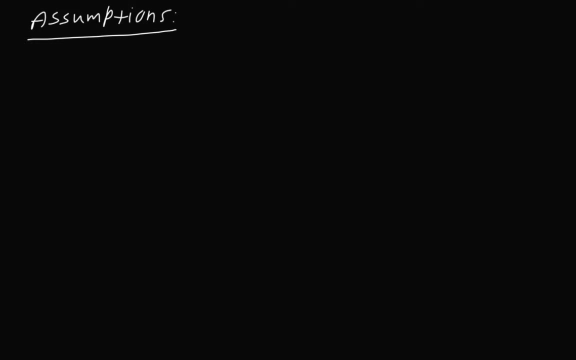 we should define our variables and assumptions. then, objective B- number of blue whales and F- number of fin whales. GB and GF growth rate of blue whales and fin whale population respectively. CB and CF: effect of comparison on blue whales and fin whales respectively. Now assumptions before I. 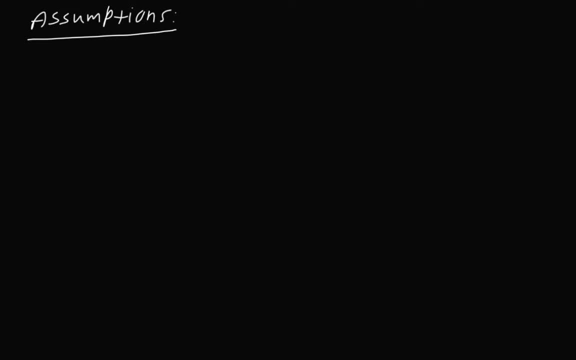 explain the assumptions of the example, Let me give an equation. We use this equation for the growth rate of population, P equal RP times 1 minus P over K. So R is the rate at which the population would keep would keep growing in an unlimited environment. 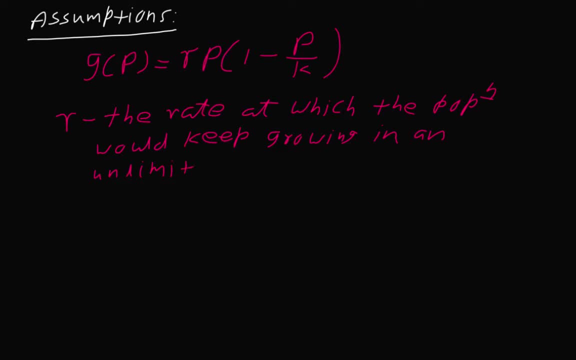 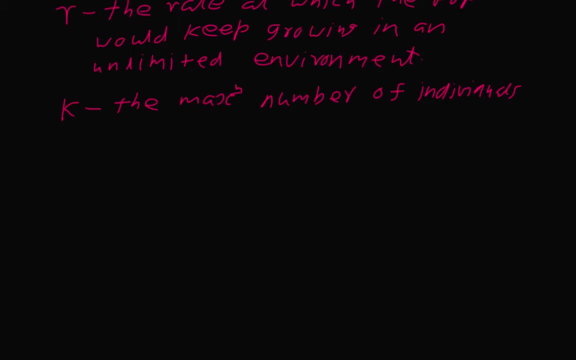 environment right And K. K is the maximum number of individuals that the given environment can support. The maximum number of individuals, Individuals that the given environment can support. We need this equation. for this example. We use GB for the growth rate of blue whales population. 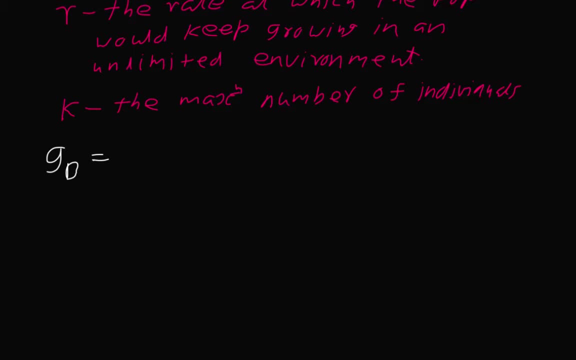 So let me write down an equation for this. So, according to the above equation, our r equal 5%. you see in the example, the intrinsic growth rate of each species is estimated at 5% per year. So therefore r equal 5%, which is 5%, which is 0.05, and k for this case. it's explained. 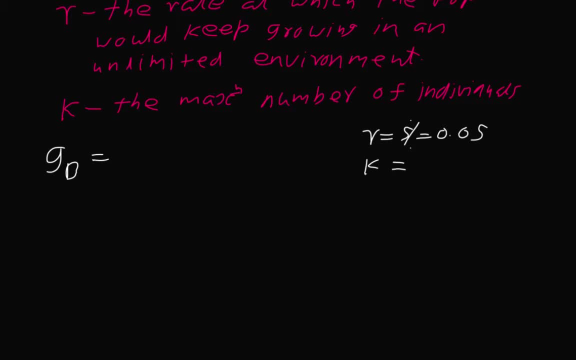 the example, the environmental carrying capacity is estimated at 150,000 blues. okay, 150,000 is the k, So now you can plug these numbers So 0.05,, so P. we use here, B, the blue whales population. therefore I will use B. 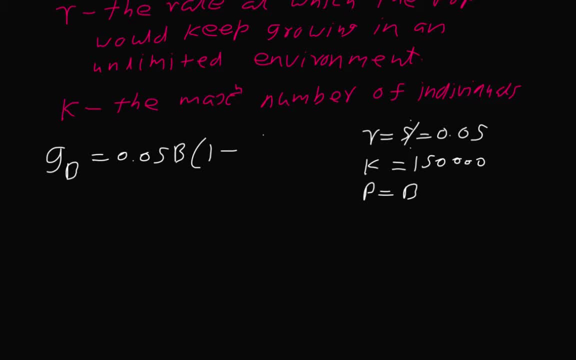 Then 1 minus B divided by 150,000.. So same thing we can write down for the GF, for the fin whales, this one 8%. Let's read the example again: It's 8%, which is 0.08.. 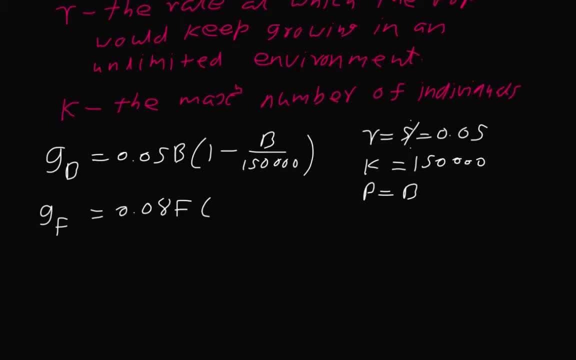 Then F, 1 minus 0.08.. F, what is the maximum? 400,000,, therefore 400,000.. So these are the two assumptions and also CB effect of competition on blue whales. so and the pin whales, both must be equal. so we can write down, I use the alpha: is the? 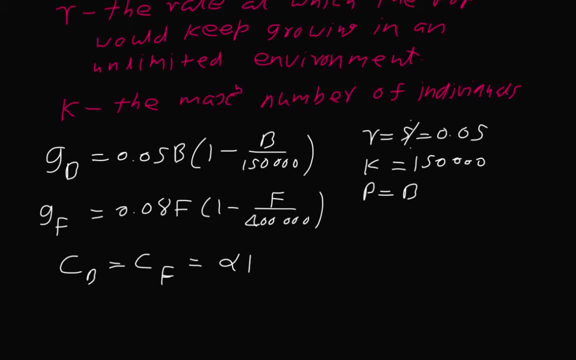 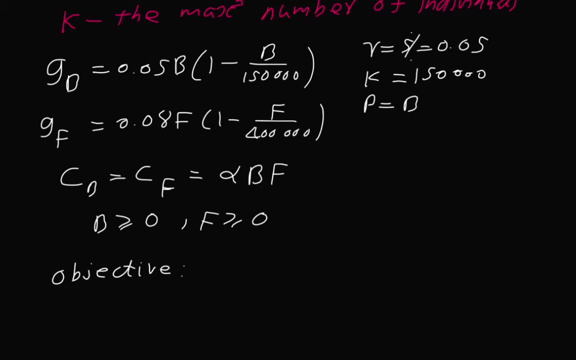 just a positive real constant. so we can write down alpha times BF. So you know very clearly: B greater than or equal 0 and F greater than or equal 0. Then objective determine whether dynamic system can reach stable equilibrium starting from B equal 5000.. 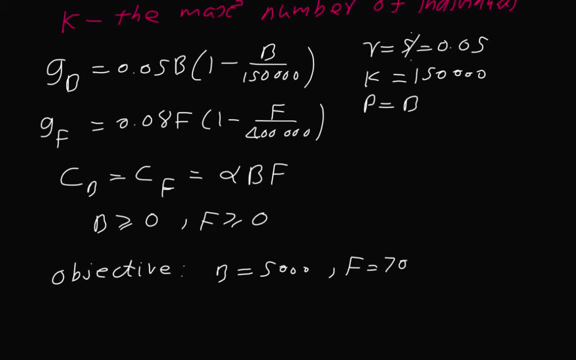 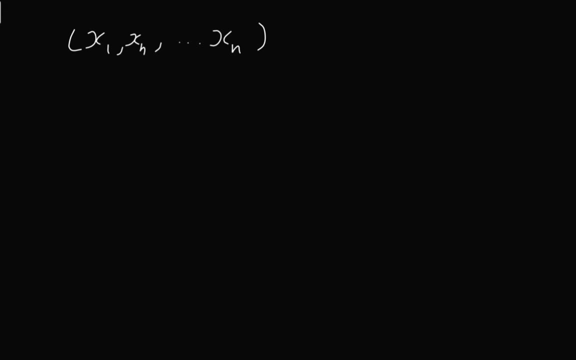 Okay, F equals 70000.. Now step two. step two is to select the modeling approach. We will model this problem as a dynamical system. So, like last time, we consider n state variables, then we do have functions F1 to Fn represent. 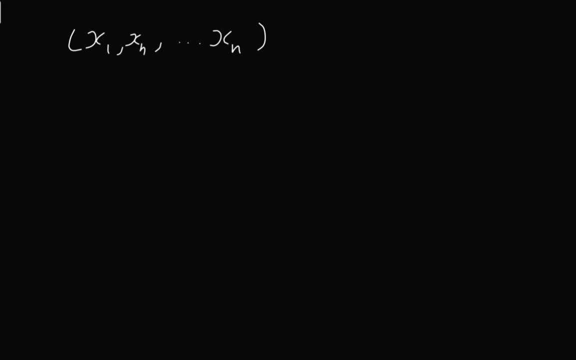 the rate of change. So I will write down same function, F1, X1, Xn. this F1 is the rate of change of variable X1. Therefore you can write down dx1 over dt rate of change of the variable X1.. 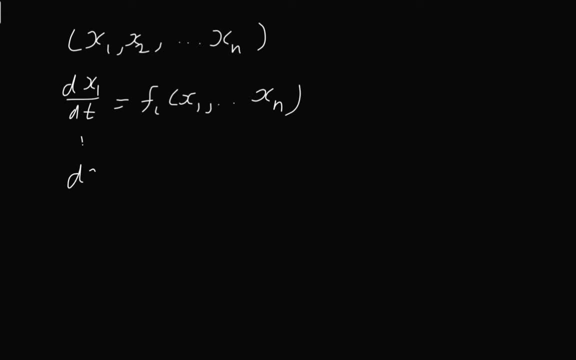 Similarly, you can write down up to n: dxn over dt Dxn. Now multiply x1 over dt fn, x1, xn, n differential equation, actually a system of differential equation. So you know, x1, xn is in S, S is a subset of Rn. 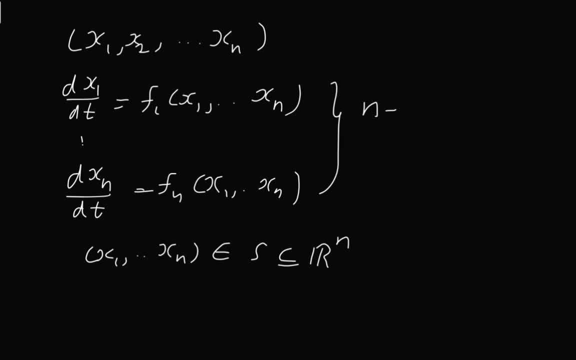 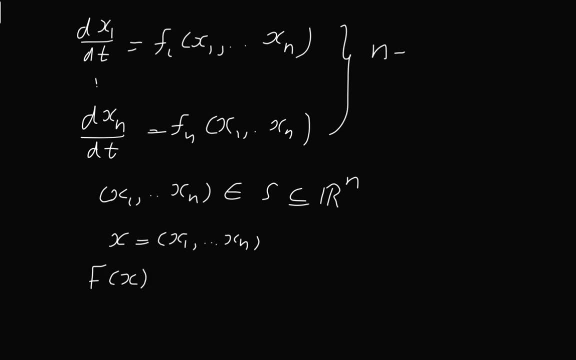 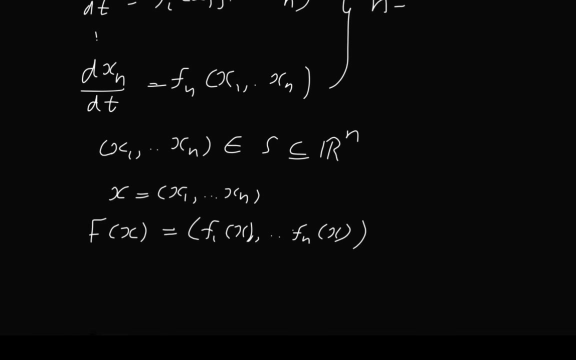 You can write down the point x, x1,, xn, fx equal f1x- fnx. Then the dynamical system equation can be written: dx over dt equal fx, Which is f1x- fnx. The points where fx equals 0 are the equilibria and we will pay special attention to the vector field nearby these points. 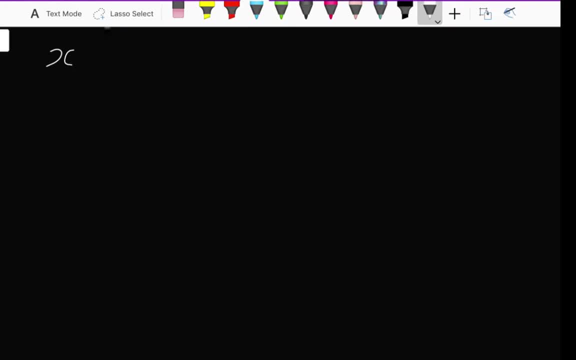 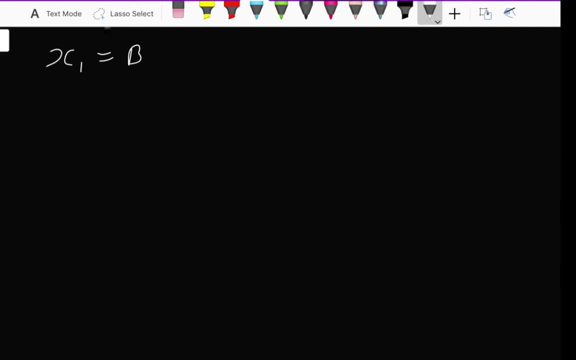 Next time we use x1 equal b and x2 equal f, Then we can write down the functions x1, prime equal f1, x1, x2.. f1 represent the rate of change of x1.. According to our assumptions, you can write down: f1, gb. 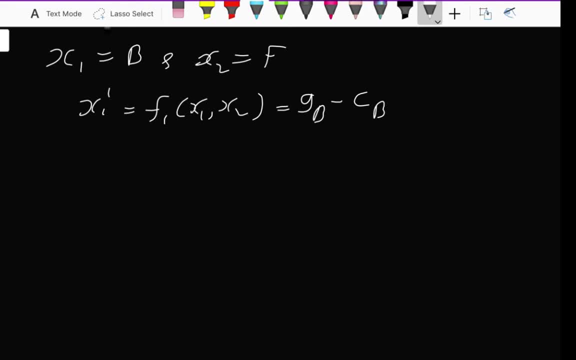 gb minus gb. Once we plot the x1 and x2, gb can be written 0.05.. x1, 1 minus x1 divided by 150,000.. You can write the gb alpha, x1, x2.. 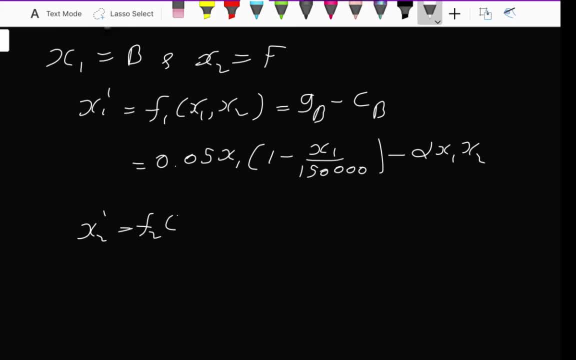 x2 prime, which is f2, x1, x2 can be written gf minus cf, So equation should be 0.08x2, 1 minus x2 divided by 400,000.. minus alpha: x1, x2.. 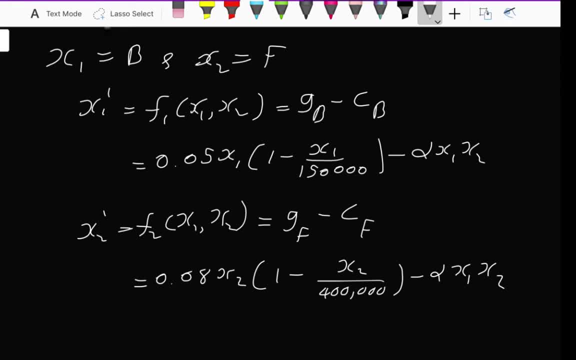 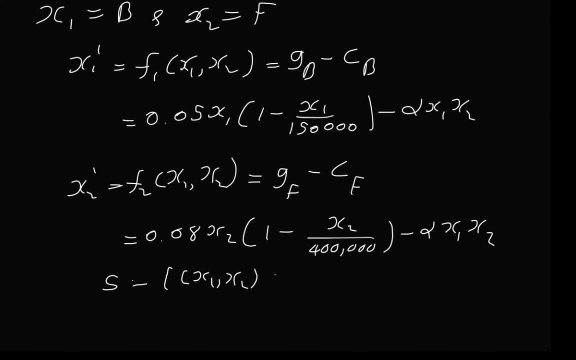 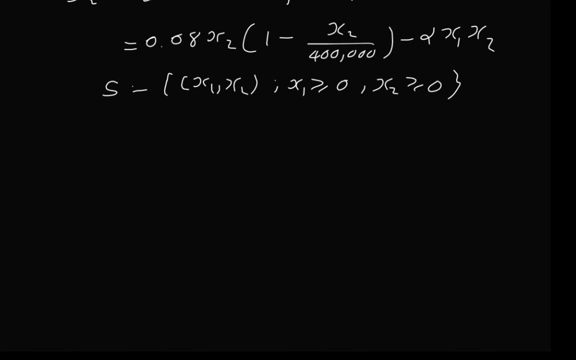 So you know the state space, which is s equal x1, x2, because we do have only two variables: x1 greater than or equal 0, x2 greater than or equal 0.. So next is step 4, which is solve the model. 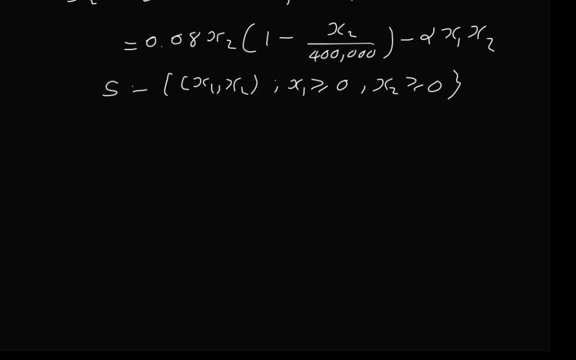 So how do we solve model, As I mentioned before? So we use the graphical method. Let me draw the graph of pinwheel versus blue wheels, So x2 versus x1.. If you consider the graph, f1 equals 0..